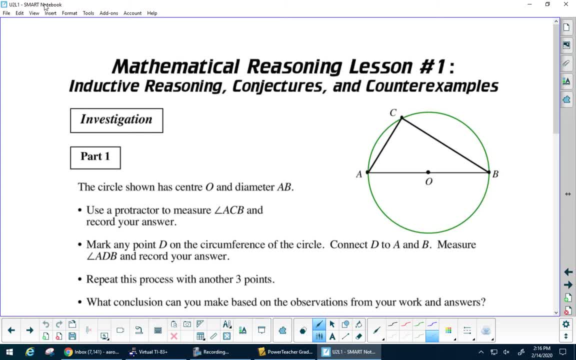 So it's logic, It's thinking before you and have you ever just got in any lineup? And then you look at the other one just moving and you're like I didn't even think about this, Like it was stupid, Why did I get in this lineup? This one's full of people that have huge carts and there's probably going to be three price checks, and you know, and look at that line moving. All those people just had a few things. okay. And that's when you learn to get a little smarter and get into the right lines. 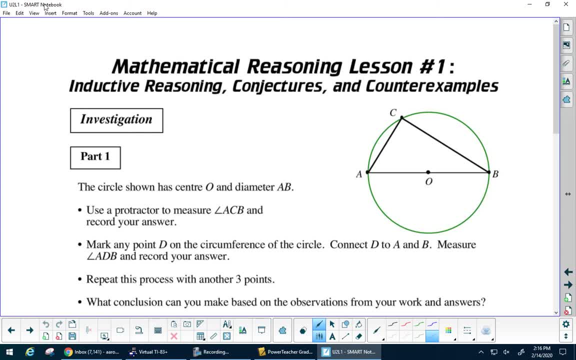 Versus a right line, versus not at all right. So today we're going to be learning about three things: Inductive reasoning, conjectures and counter examples. okay, And you would be surprised how many of you know these already, but you maybe didn't know that was the word for it. 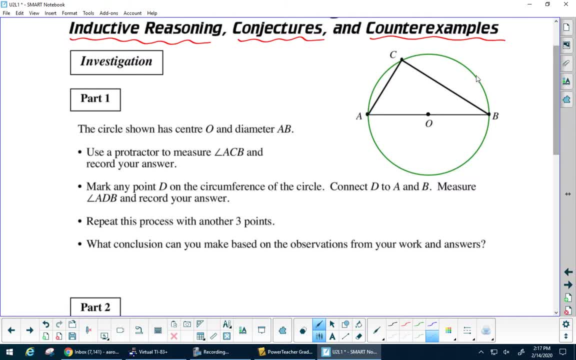 Let's just look at this. This is a diameter Cuts your circle in half. And do you know that on your diameter, if any time you take so from A to B, you go one place over and then back, it will always make a 90 degree angle. 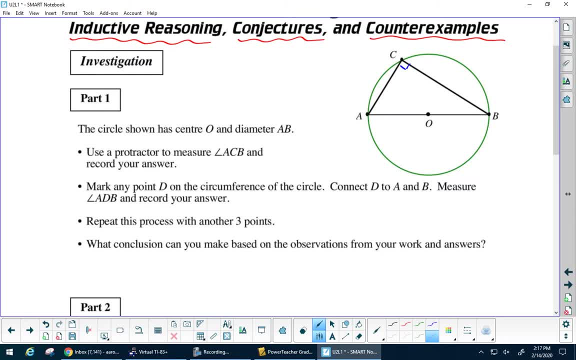 So what does that mean? That means okay, so I should be able to go like this, then This side and then down here And, believe it or not, it does make a 90 degree angle. You could do it over and over again. get your protractor out and you will find every single time, and then you could come down here and do this one. you could try this one and, believe it or not, every single time will make a 90 degree angle. 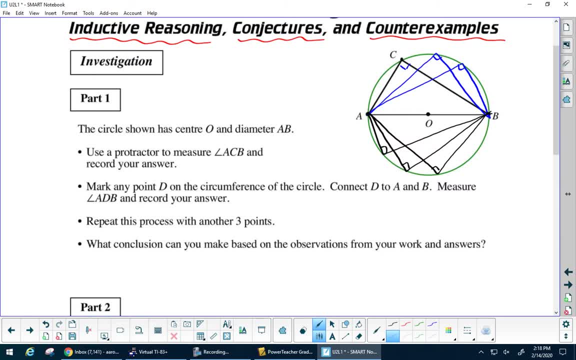 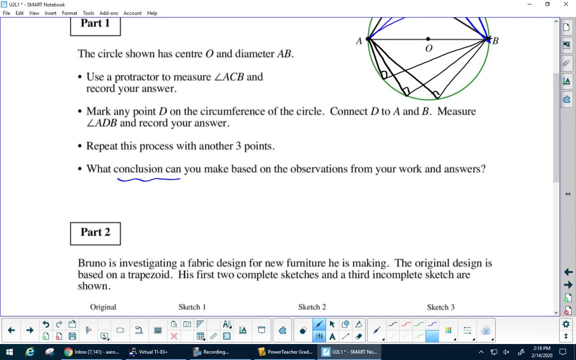 So the question or the conclusion you can make is that any angle made on the circumference of a circle, whose arms, I'm sure you wouldn't think to do it this way, but whose arms pass through the endpoints of its diameter, is always 90 degrees. 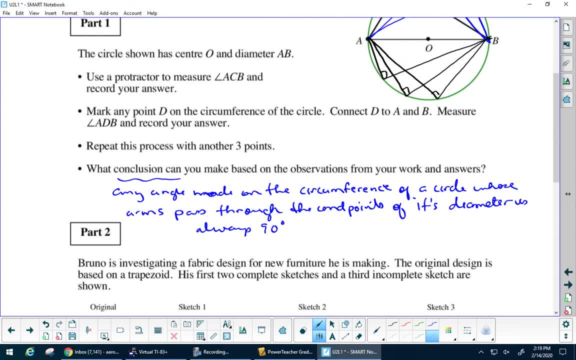 Okay, now you want to try to crop a load of times to make sure it works. Not just one time, Okay, not maybe even ten times. Maybe you've got to do it many, many, many, many times to see if it fails. 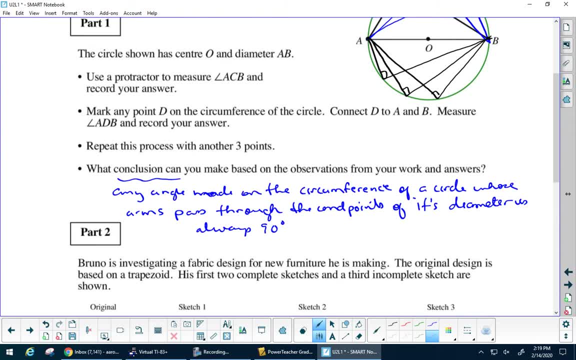 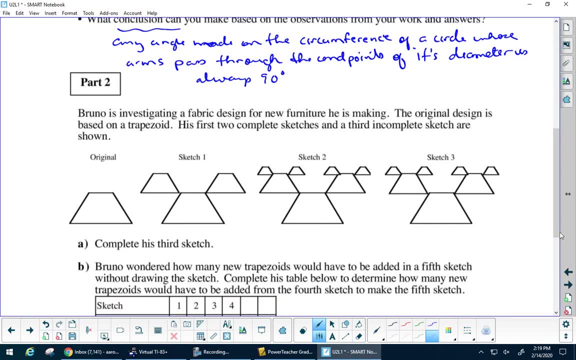 Until you can say you know what. that's true all the time. Okay, now Bruno's investigating his fabric design for new furniture he's making. The original design is based on a trapezoid. His first two complete sketches and the third incomplete sketch are shown. 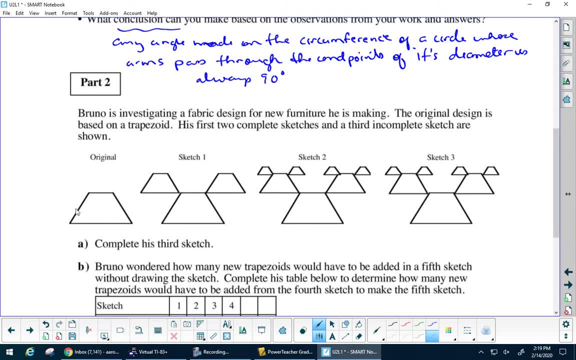 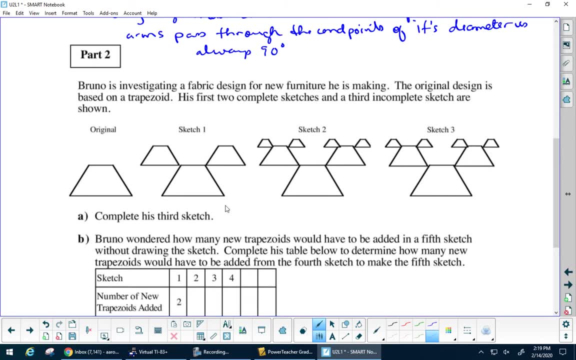 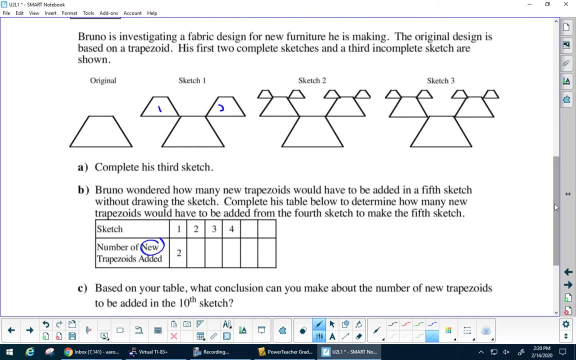 Okay, so here's a trapezoid. So in sketch one all he did was add two new trapezoids- One, two, And in the second sketch he added trapezoids. if you can see, he added trapezoids to each one of these two to get one, two, three, four. 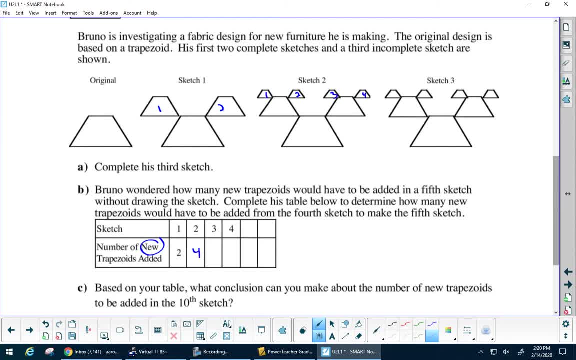 So in sketch two there was four. Now in sketch three, right, he's going to add trapezoids to every corner. So in sketch three he's going to add trapezoids to every corner. And how many are there? 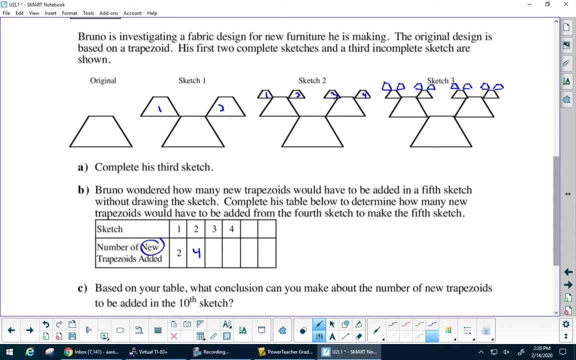 How many new trapezoids did we get? We're just looking for the new ones. How many new ones? Count them up: One, two, three, four, six, seven, eight. now do we? it's a lot of work drawing all those trapezoids and look how much, how bad mine suck on top of that. so they're even. 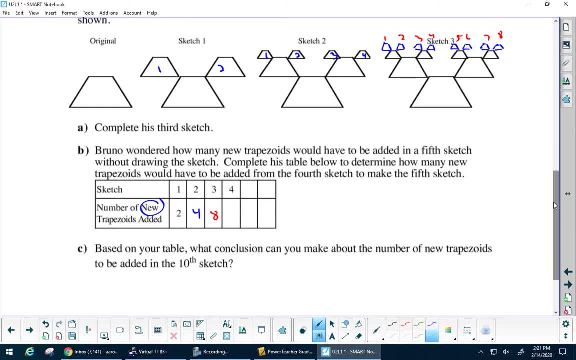 ugly trapezoids. is there a better way? how many do you think would be in the fourth? 16? how'd you get that? see how it's been doubling. so at five there should be 32, and at six there would be 64. there's even a better way to do it. 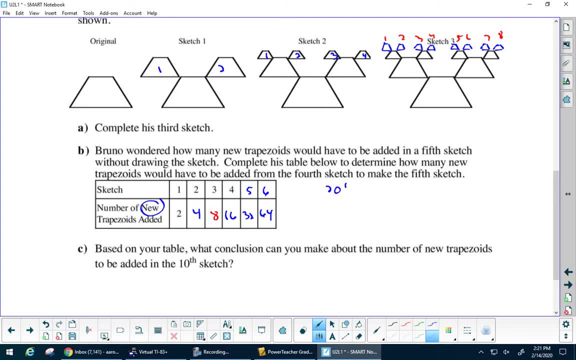 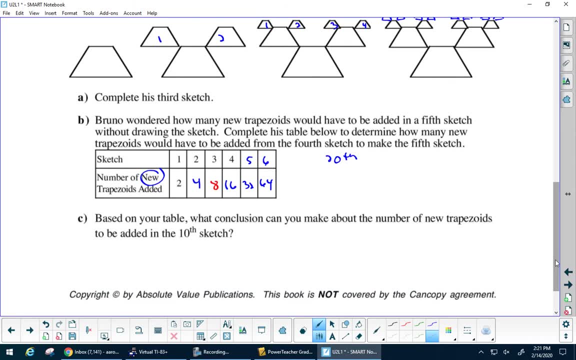 because what if I wanted the 20th? then you're like, ah, that sucks, I got a lot times two times two times two. but there's a better way. what is a way you could use these numbers to get these numbers like: what can you do to two to get four, or how could this okay? 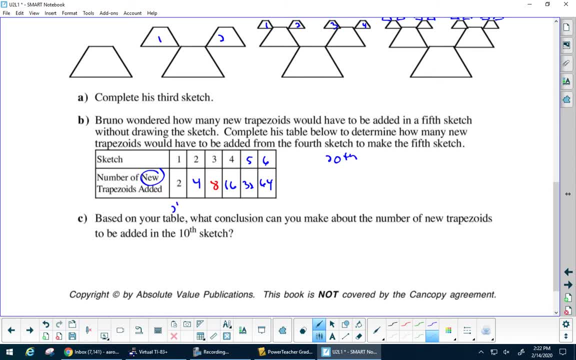 so I'm going to show you a little trick. this is like two to the one, this is two to the two, this is two to the three, this is two to the four, this is two to the five, this is two to the six. so to find the 20th, I would do. 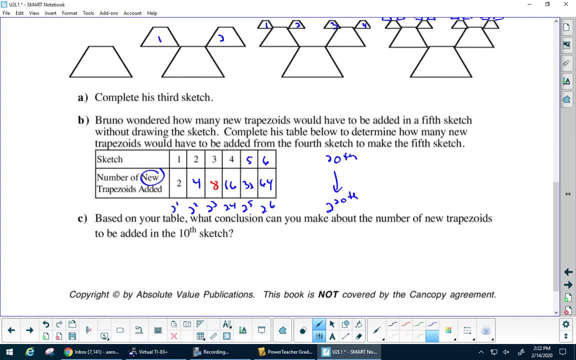 two to the 20th. so because it keeps doubling right. so you got two and the next one's two times two, the next one's two times two times two, the next one's two times two times two times two. so that's how you get to the one to the two. 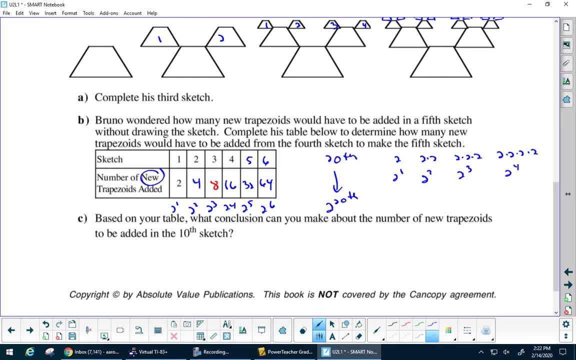 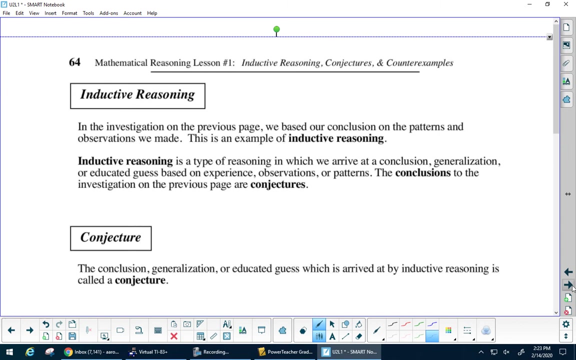 two to the three, two to the four right. so, based, what conclusion can you draw for the tenth sketch? the number of trapezoids should be two to the tenth or 1024. okay, so, believe it or not, what we've been using is called inductive reasoning. 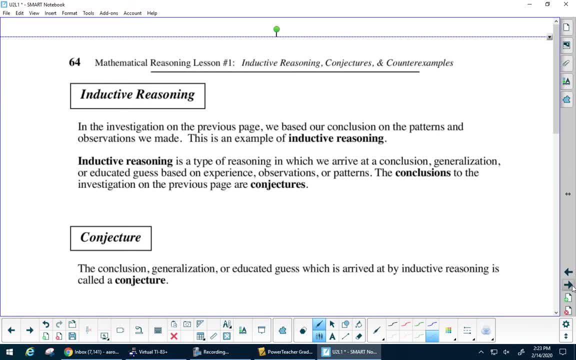 now, what is inductive reasoning? okay, inductive reasoning- let's just read along right here- is a type of reasoning in which we arrive at a conclusion, generalization or educated guess based on experience, observations or patterns. so it's based on experience, observations or patterns. the conclusions are called. 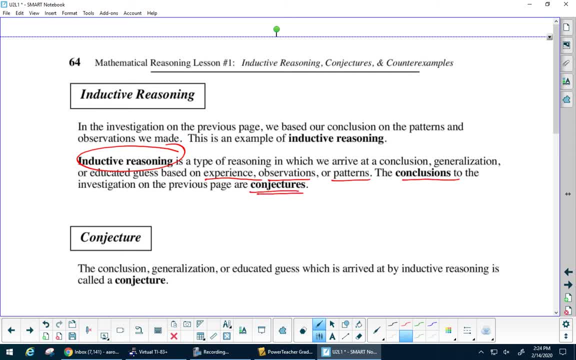 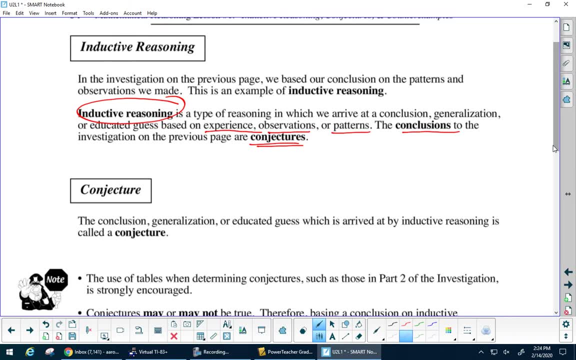 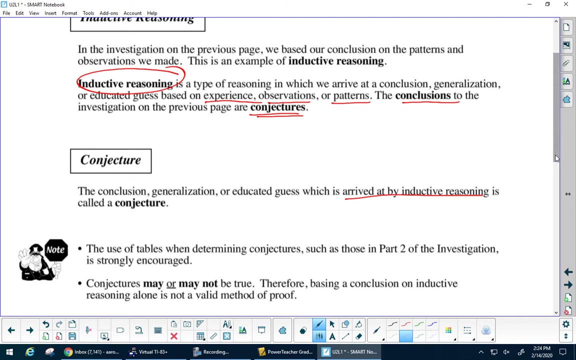 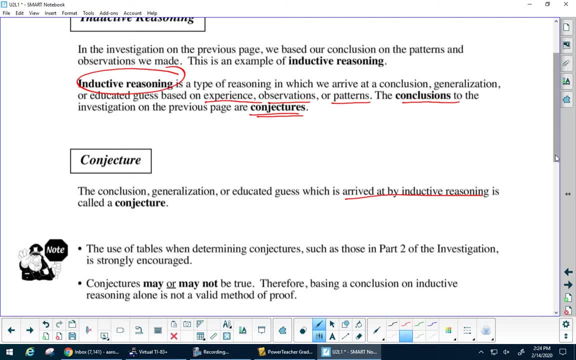 went to this little store on the corner and it was closed. okay, the next Sunday you went to that store and it was closed. and then someone says to you: yeah, I'm gonna go to that little store on Sunday you go, it'll probably be closed. that's inductive reasoning. now it may not always be true. maybe for those two Sundays that person was. 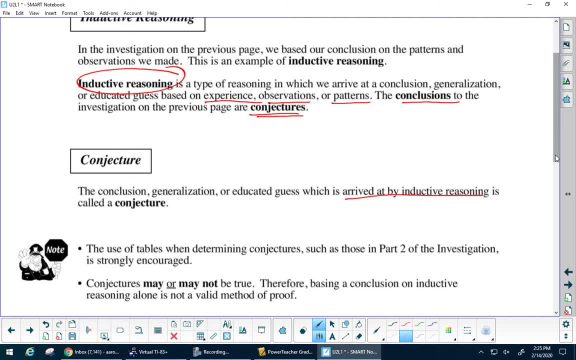 and and maybe they're back, and now it's going to be open sunday. or you walk into a like a computer lab, and the first computer's a mac and the second computer's a mac and the third computer's a mac and you go: this must be a mac lab, it's all full of uh apple. 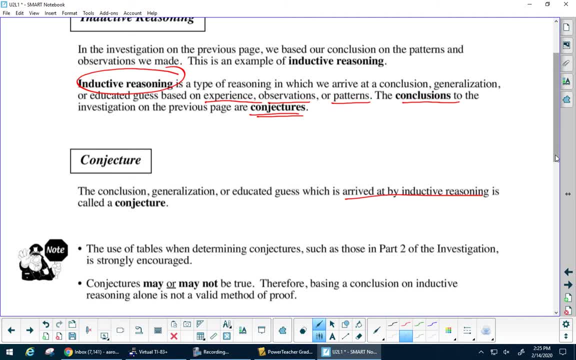 but maybe there is some pcs in there, right? or you lend your buddy money. he doesn't pay you back. he asks you for more money. you lend it to me, doesn't pay it back. the third time he asked to borrow money, you say no. why you're using inductive reasoning now? is it for sure? true, he won't pay you back? is it a guarantee? 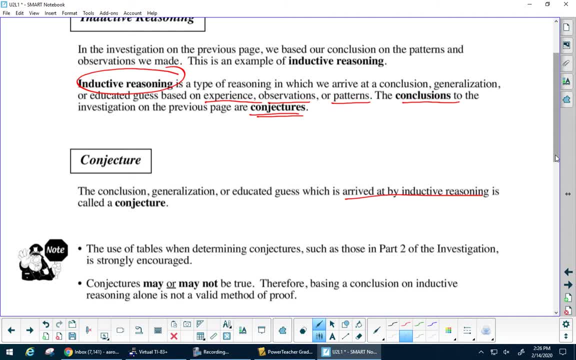 would you bet your life on it? no, but we use inductive reasoning all the time. you just have to realize that it may be false. okay, like you know, the last time i had a math test, i had a chicken that night, the night before and i did awesome. and then the next time i had a math test, i chickened that night. 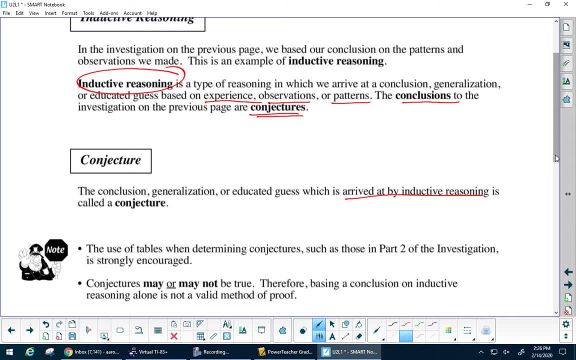 and i did awesome. so from now on i'm having chicken before i write a math test and sometimes we've got to be careful about that. i'm not going to be able to do that. superstitions are based on that. a lot like hockey players a lot. 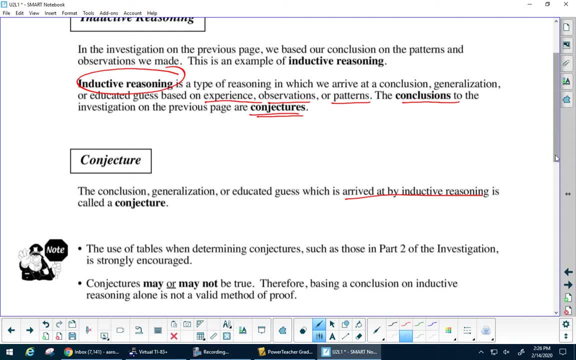 of them have superstitions that they always have to put on the right pad first or they always have to be putting on the left skate first, always, and they'll find out the times they don't. they play crappy. so by inductive reasoning they say: if you don't put your left skate on first, you will have. 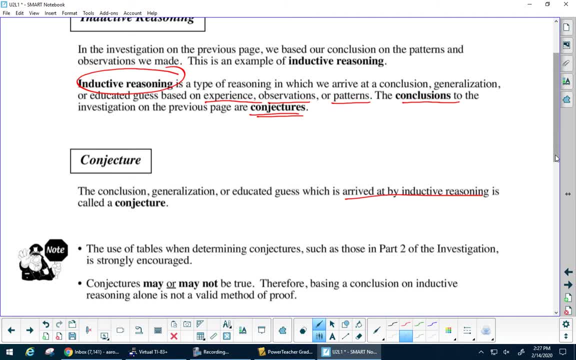 a crappy hockey game. so is all inductive reasoning based on fact? no superstitions. uh are based on history of inductive reasoning. uh, you know there is uh diseases. you know how diseases are contracted. uh, you know we got to make sure we wash our hands. we got you know. that's all based on. 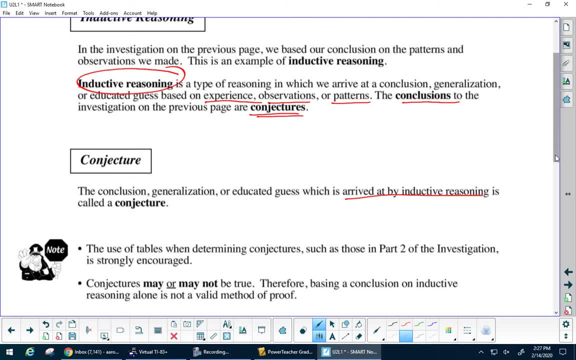 inductive reasoning. they found that if you wash your hands, that the flu is not spread as wide. okay, now just remember that that conclusion or generalization is called a conjecture. now i gotta ask you a question here. if your parents say: you know what, i'm sick and tired of you in this house, you 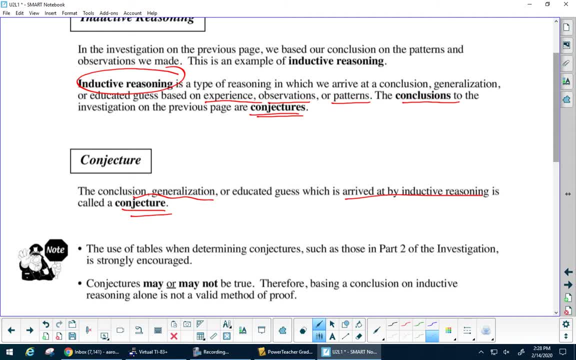 never, ever clean up around here, and it makes me mad. how have you? what would be something you could say to that that could stop that conjecture you could clean? yeah, that wouldn't stop the conjecture. you would actually keep that true, you could clean. or you could say: 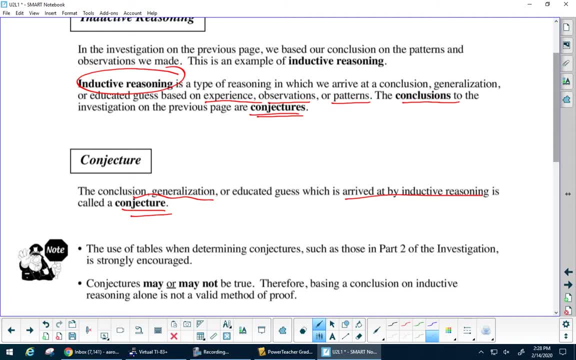 i cleaned up the house last tuesday, okay, i cleaned up the house last tuesday, okay. and if that's true, or three people didn't clean up the house last tuesday, okay, and if that's true. or four people didn't clean up the house last tuesday, ok, so its not true. all of that is totally conflicted, ladies, ladies and gentlemen. so what are the customer side to the truly i clean up the house, community, and we will be rememberfel pagan life better again. αrop наш HR. 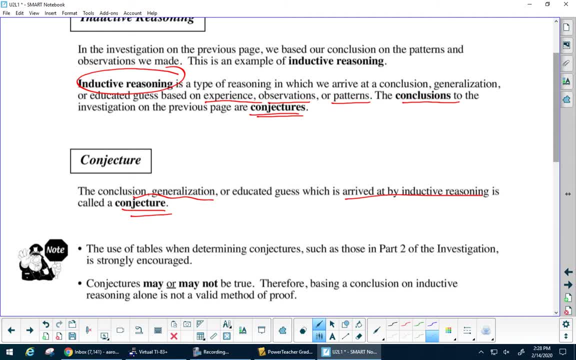 that's true. of course we're gonna. you have now disproved the conjecture hundred percent. that's all you need to do in life and in inductive reasoning or conjectures. you just have to give one example of where that is not true and it throws it out. same with the court of law, okay. 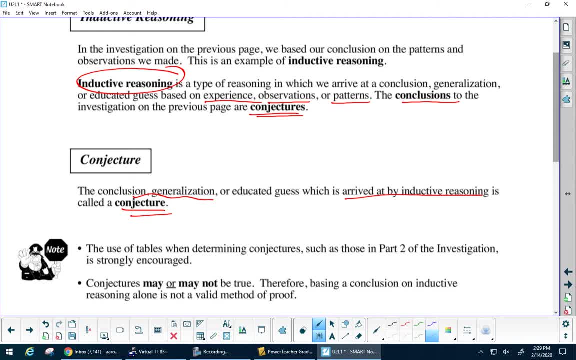 if you can just give one example where that is not true, then it's considered never true. okay, so if your parents say: you know what? I'm sick and tired of? you're just here all the time. you don't do any work. you all you do is freeload this, this, this, and you're like: but I like clean up the whole. 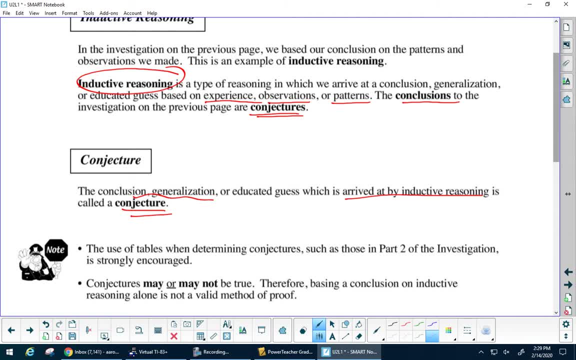 house last week. that means: and that's not true. if that was a court of law, the judge would say: you well, is that true, mom? did she clean up? yeah, she did, okay. well then, this court, this case is over. you can't make that statement. it's not true. and if your buddy is like and you're like 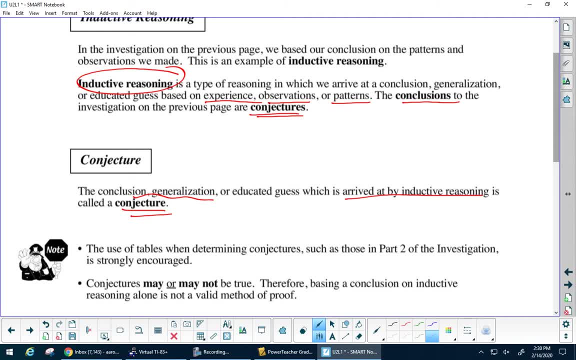 I'm not lending you any more money because you never pay me back. he's like: I paid you back like last week. right, you may not lend him the money, but that's not true. you, if that was in a court of law, you would lose. okay, if you can prove that that statement is false by one counter example, then it is false, okay, and 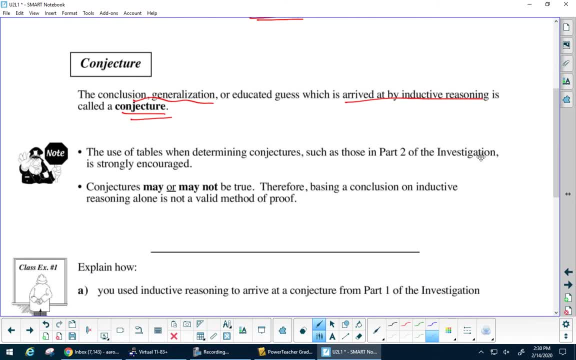 we're going to talk about that in a bit too, so this is super important. you guys, conjectures may or may not be true. in fact, some are complete lies. you know a lot of um. sometimes people just get these ideas in their heads because maybe their parents told them that right um anytime, any there's racism or things like that people get. 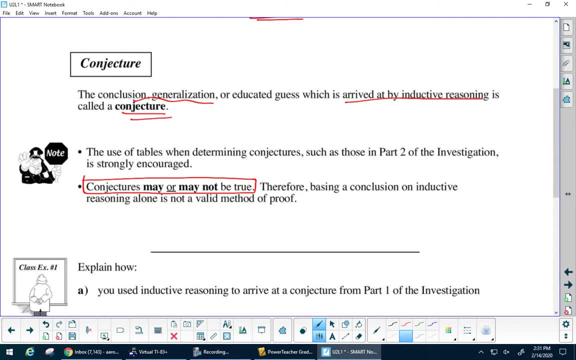 stuff put in their head. that's not even true, but they just believe it to be true and they act off it. okay, that's what racism is: discrimination, right? people discriminate against another culture, right? because, oh, they're not as good as us. well, where did you learn that? I was taught that, and I believe it to be true. 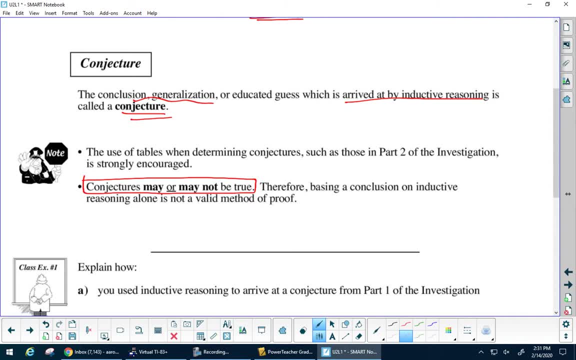 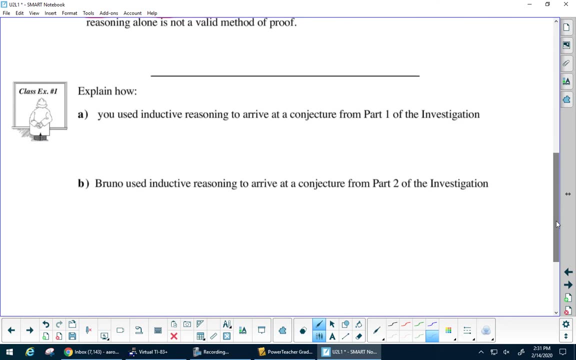 right, and the only way to disprove that is to show many, many, many examples of how that race or that culture that's not, that's not true and that's the only way we get rid of that racism and discrimination. okay now, um, if we- because we kind of already did that- now we're going to talk about counter examples. 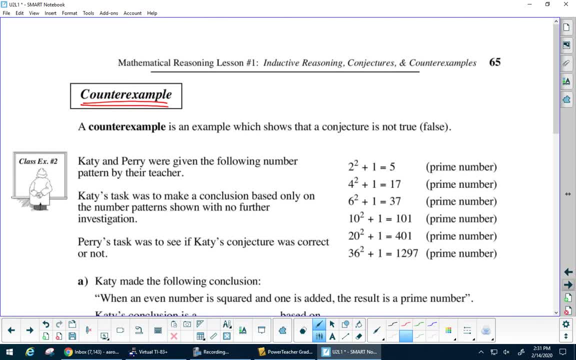 now this is super important. if a uh a conjecture will be true unless you can provide one counter example, you don't have to do 10.. it's just one and it proves it to be not true. so a counter example shows the conjecture is. 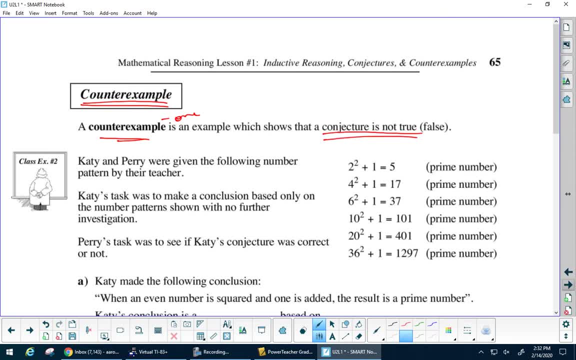 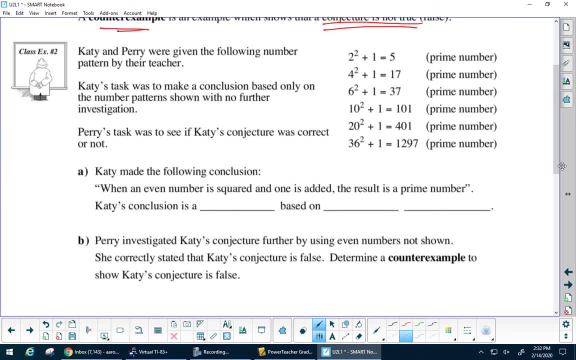 not true aka false, okay, so I want you to look at this one: Katie and Perry- it's kind of funny that they use those two names. I wonder if it was a coincidence. we're given the following number pattern by their teachers. Katie's task was to make a conclusion based on only the number of patterns shown and 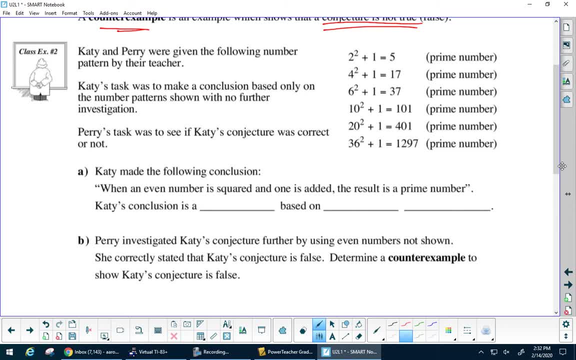 no further investigation. so she found that from this, two squared plus one equals five, four squared plus one equals 17.. six squared plus one equals 37, 10 squared plus is 101, 20 squared plus one is 401, and 36 squared plus one equals 297.. now, if you look at all these, they're all prime numbers. now what's the prime number? 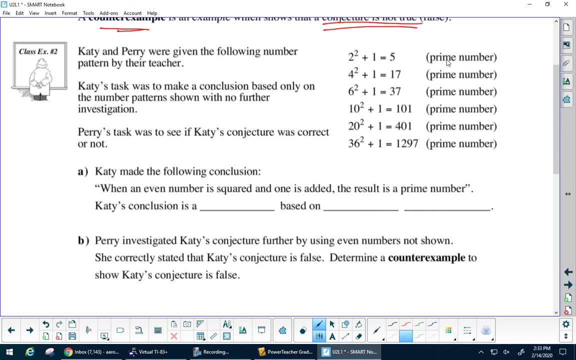 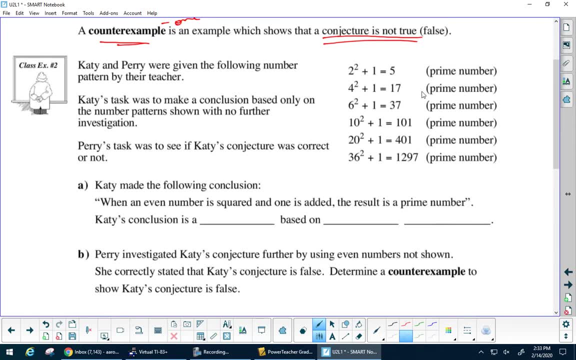 anyone know math 10.. it can only be divided by one and itself, so like six. well, six would be one, all right. all of the factors would be one, two, three and six. so two times three is six, right, but if I gave you five, what times? what equals five? 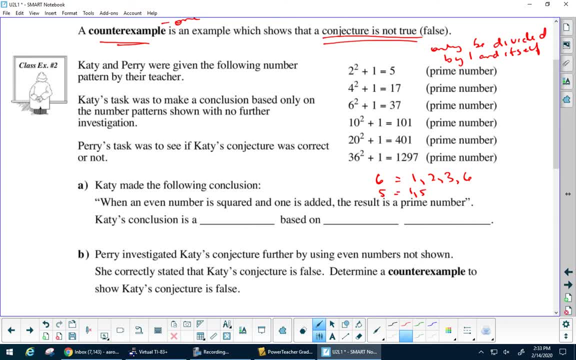 well, only one and five, so it can only be divided by one and itself. so one times five is five, that's it twelve. I can go one times twelve, I can go two times six, I can go three times four. right, that has more than one. so she had to provide a conjecture based on this. they did, she didn't. she's not asked. 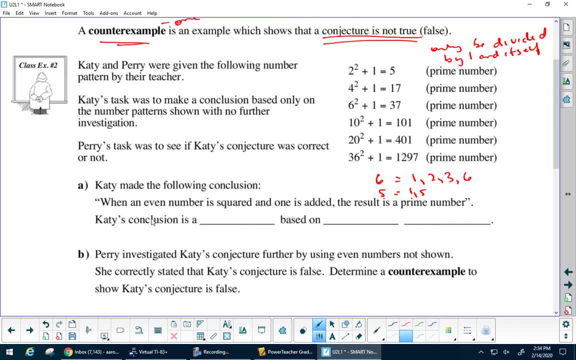 to come up with the counter if it's true or not. but her counter, her conjecture, was: an even number is squared and one is added, the result is a prime number. so Katie's conclusion is a conjecture based on inductive reasoning. so you can have: 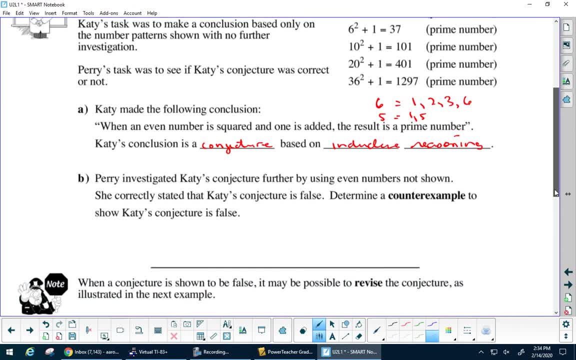 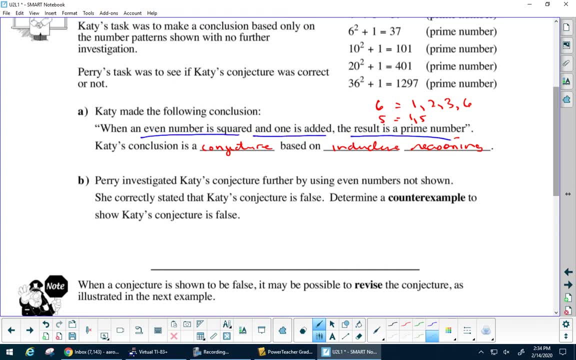 a constant with an even. Now, what's your conclusion? When an even number is squared and one is added, it'll give me a prime number. Is this true? You can't say no unless you can give me a counterexample. What's that? 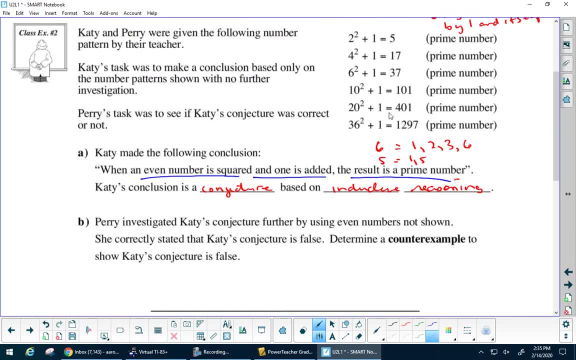 No, all of these are prime numbers. Every one of these is correct and true Is there. can you give me an even number, squared and one is added and the result is not a prime number? Because if you can't, then this remains true. 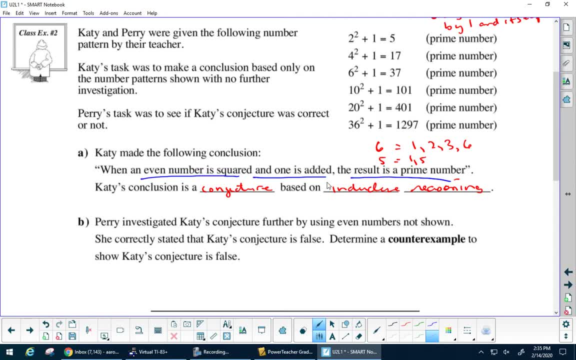 And that's what every single lawyer does: Find something to disprove, especially any defense client. Anybody that has been charged with something gets a defense lawyer, And your defense lawyer is very good, But at finding one counterexample. If they find that one counterexample, they get you off 100%. 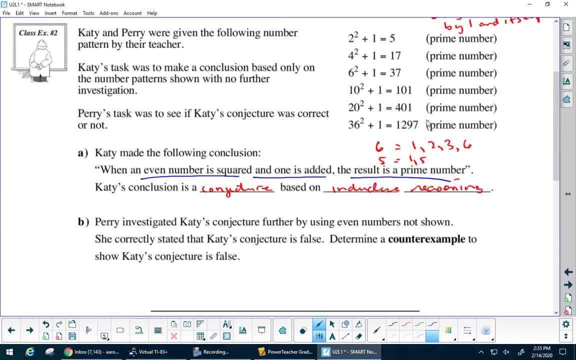 So 18 squared. Okay, let's go with the smaller one: 18 squared, 8 squared plus 1.. That's 64 plus 1 is 65.. Is 65 a prime number? No, this is called a composite number. 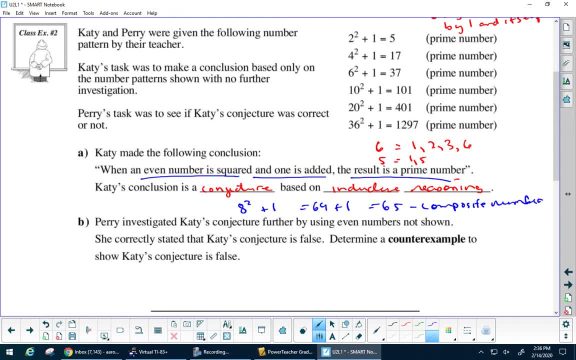 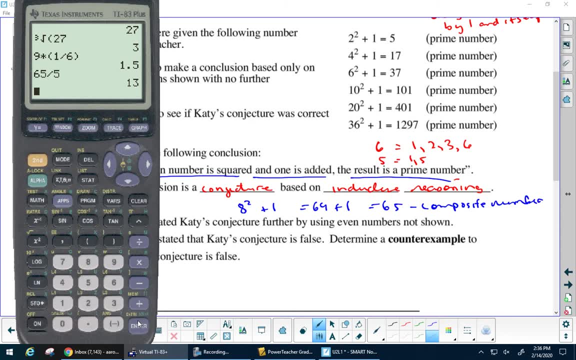 Because it's more than 1 in itself, Because 65 divides by 5,, right? If I do, 65 divided by 5, it's 13.. So you can divide by other things than just 1 in itself, right. 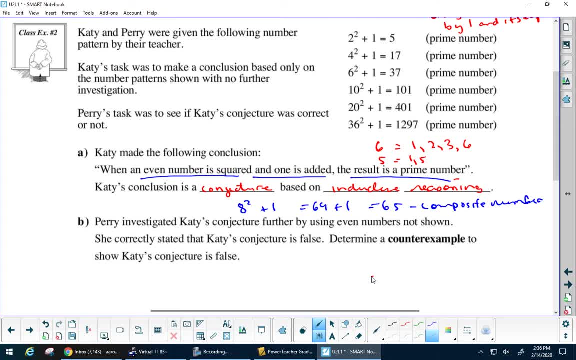 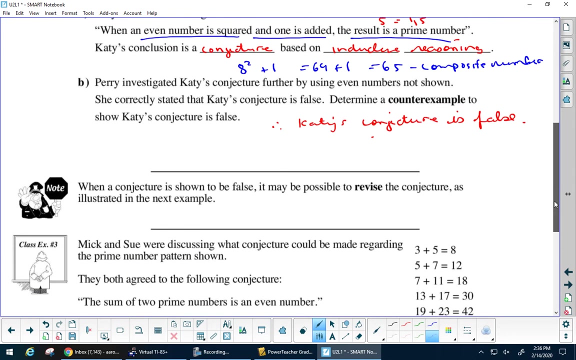 So this proves that this conjecture is false. Therefore, KD's conjecture is false. KD's conjecture is false. So if someone tells you every person that works for us is completely honest, okay, and if you catch one person stealing, you get to say back. well, there you go. I just 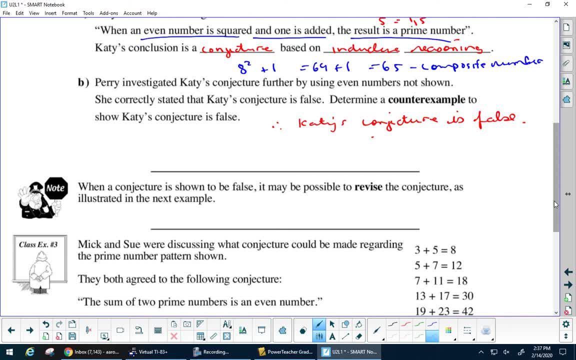 disproved your conjecture. every person working for us is not honest. we need to be watching. okay, if you know some neighbors complaining that your dog always crops on their lawn and you're like: my dog has never, ever cropped on your lawn. meanwhile you look down and the dog cropped on the lawn. I 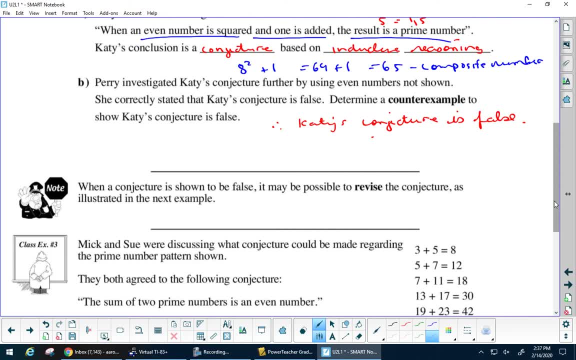 think you kind of look like a fool at that point and it looks like he's done it all the time right, and that's the bad thing about ever making a conjecture that is false is that you feel like an absolute fool when somebody proves you wrong, okay, and that's why parents don't like that. when 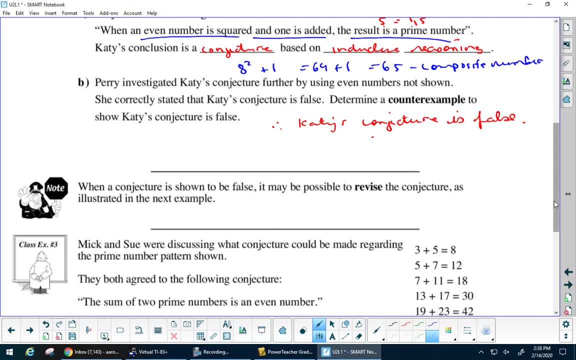 they say that your pig, you never clean up, you just expect everybody. and you give them an example, do they go- oh, that's a really nice dog. and you give them an example. do they go? oh, that's a really nice example. thanks for that. I am very calm now and cool, collected, and I am sorry for everything. 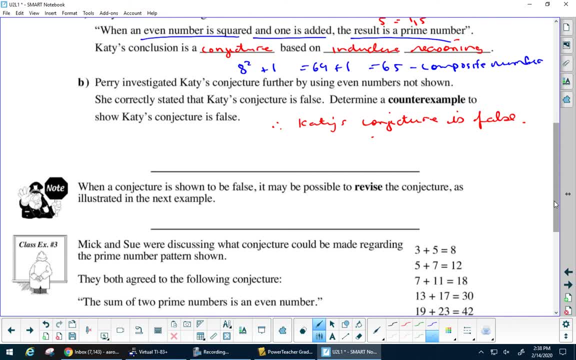 right, never goes that way, does it? so there's times that we don't even point out the counter example, because it's like, okay, okay, fine, yeah, mm-hmm, I'll just clean up, because you provide that counter example and you get in more trouble. you're talking back or your whatever, and that's. 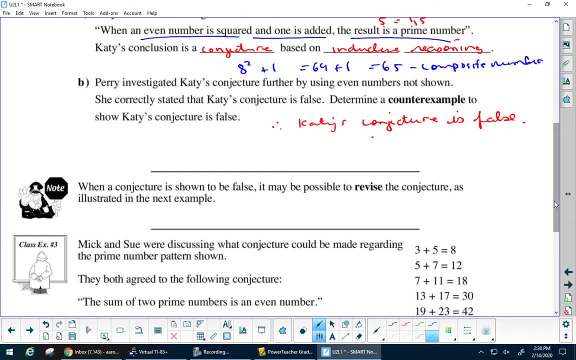 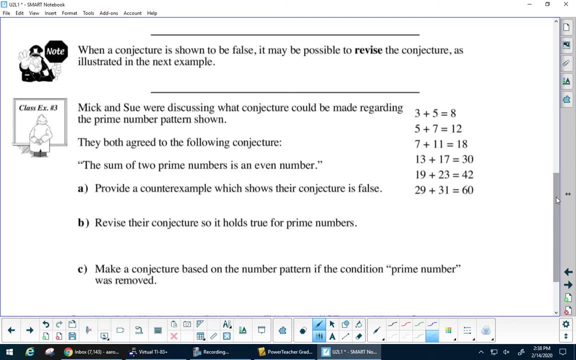 why it's, I guess, great to be a lawyer? because you get paid for talking back right now. let's try another one now this: when a conjecture is false, it may be possible to revise the conjecture. okay, because sometimes you can, because maybe your parents will say, because you'll just. 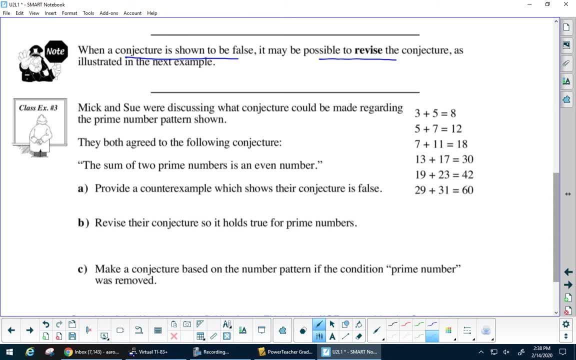 like: oh no, you remember last year on September 16th I picked up my coat. yeah, uh-huh, yeah, and parents go: no, in the last year you have not done anything. you're like i'm screwed. why did they make it right? they said never. i liked it when they said never, i've never helped clean up. but now they said: 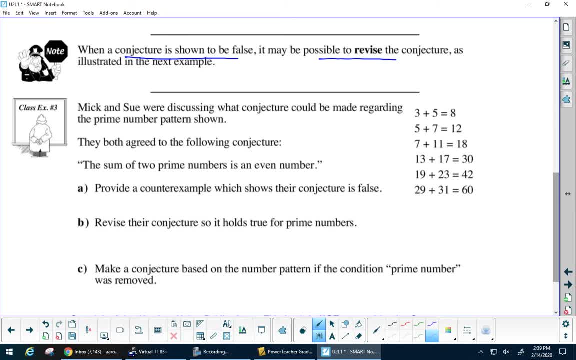 in the last year. so they revised their conjecture and now you're screwed. right now, what are you thinking? right away, come on, come up with something. come up with something that i cleaned in the last year, get it now right, and then maybe you can't, and then later you're like thinking about: oh yeah. 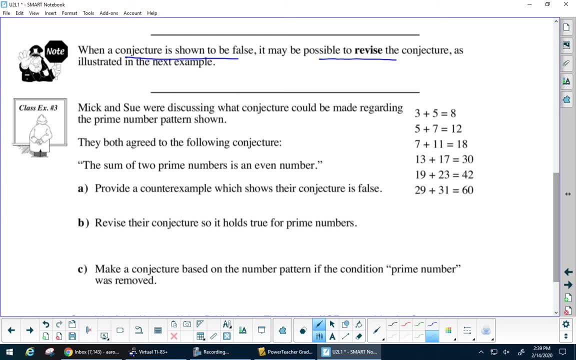 there was that time i should have said that. i wish i wish i said that right now. so mick and sue were discussing what conjecture could be made following with uh regarding these following prime numbers: three plus five. so these are all prime. three plus five is eight. five plus seven is twelve. 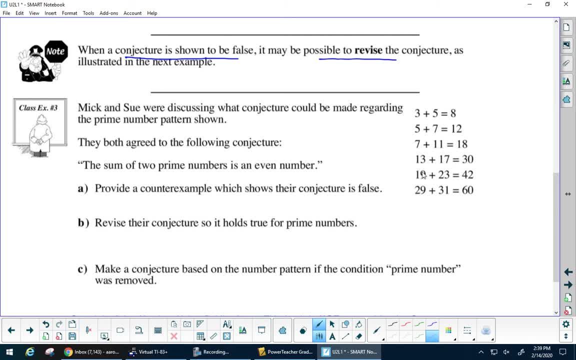 seven plus eleven is eighteen. thirteen plus seventeen is thirty. nineteen plus twenty three equals forty two, and twenty nine plus thirty one is sixty. so they both agreed. this is the conjecture that they're going to make. the sum of two prime numbers is always an even number. 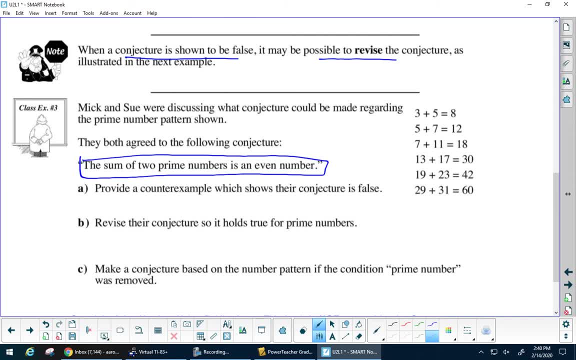 true or false. and don't say false unless you can tell me why- and that's why people who cannot find counterexamples, they fall for everything. have i got a deal for you? it will not fail right and you're not willing to like? do some research and find out. actually, it fails a lot. 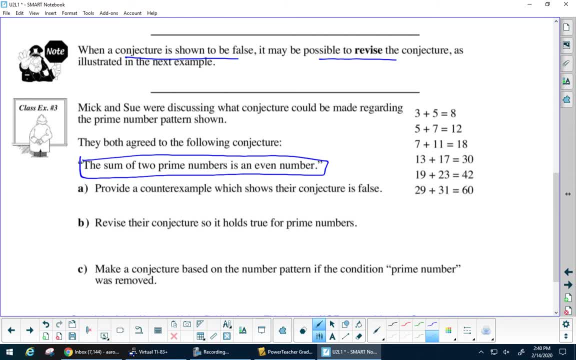 i'm not going to go into business with you, and that's mathematical reasoning. you only learned that in math. right, it's coming up with something that to say no, no, i'm good, right, but if you count, if you're not good enough at finding a counter example, then basically you have to do whatever happens. right, anybody got anything. 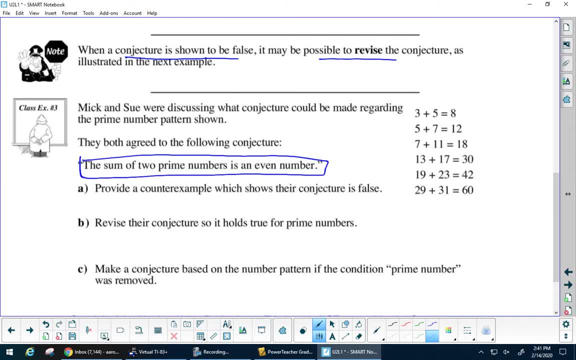 so is this true? there's only one counter example that fails: two two is a prime number, and look at: two plus three equals five. there, that is not an even number. therefore, that conjecture failed, so i'm going to go ahead and list my numbers and i'm going to count that. 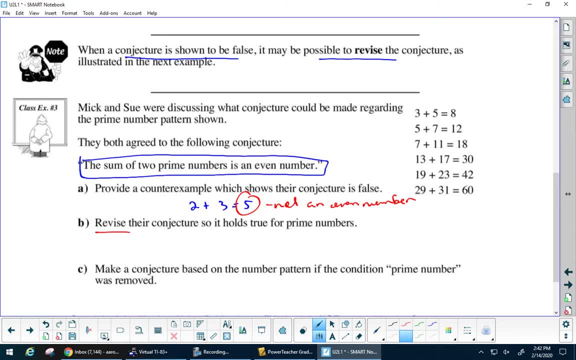 is false. so the question is: could you revise this so it holds true? right so, the sum of two prime numbers. you could put the sum of two prime numbers- maybe i'll use the word two- two prime numbers except for two. or we could say: excluding two is an even number. 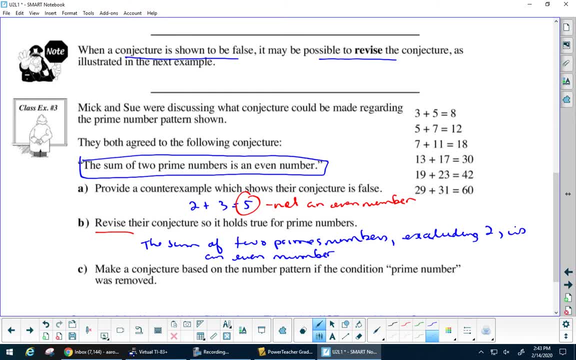 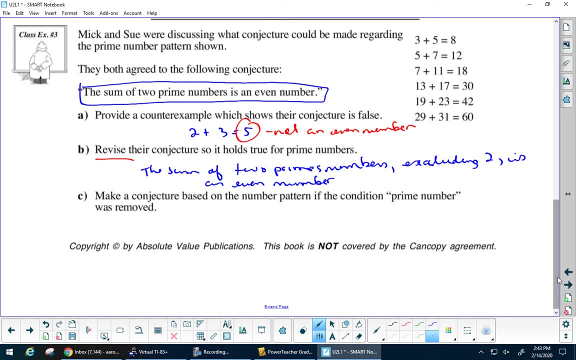 okay, now make a conjecture based on the number pattern. in these conditions, if they took away the way prime number. so if we take away the way prime number, we got rid of prime number. what could we say? that has happened here. what are all of these numbers? odds, right, so we would say the sum of two odd numbers is an. 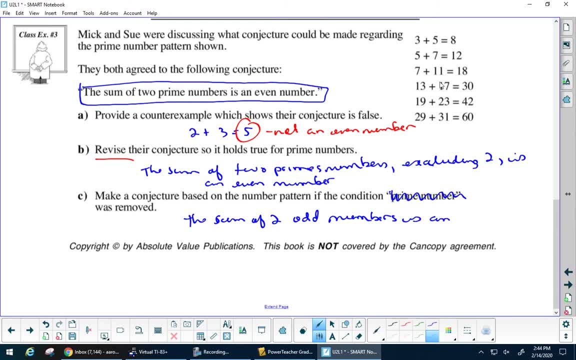 even number. and that's my favorite thing about the white boards: when two people are working together and somebody comes up with something and someone goes: wait a minute. i, that's not true. here's why- and they say, why when they're, they're in that, why territory? that means they get what's going on. 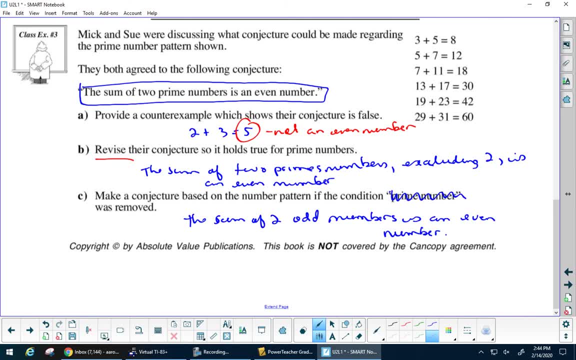 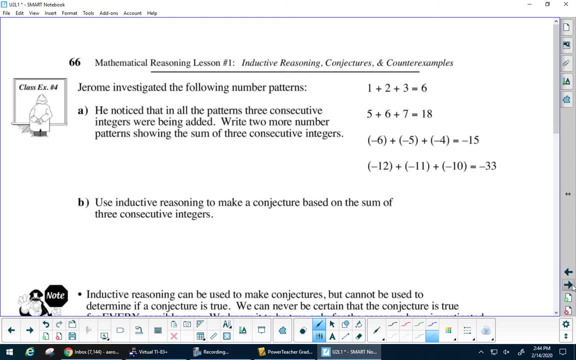 okay, now jerome investigated the following number pattern: one plus two plus three equals six. five plus six plus seven equals eighteen. and then negative six and negative five and negative fifteen. negative twelve: negative eleven: negative ten equals negative thirty three. he noticed that in all the patterns three consecutive, when three consecutive integers were added. 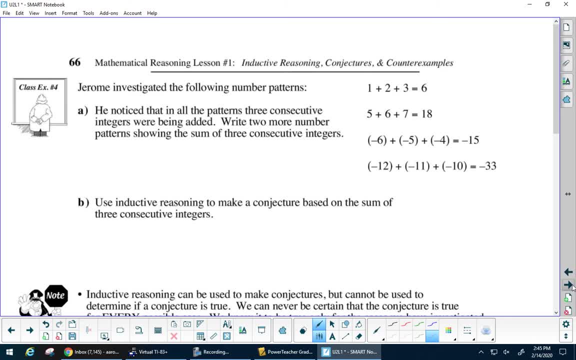 when two or more write two more number pattern showing the sum of three consecutive integers. this is pretty cool. so when you have three consecutive numbers, what's a faster way to find the answer? like like twenty-one, purely dance to regarded for sixty six. what happens in this migrant? what happens if you? 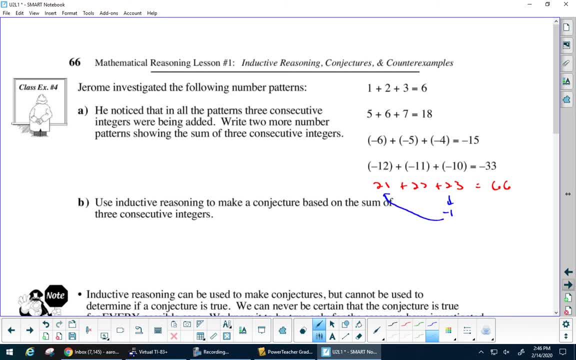 take the one away from here cannot work. we got sixty-six delhi, so this is a slate, because if i bring it over here- since this is always one less is also one more- i can bring that here. right, what would I get? 322 66. so if I just gave you this? so I want you to just 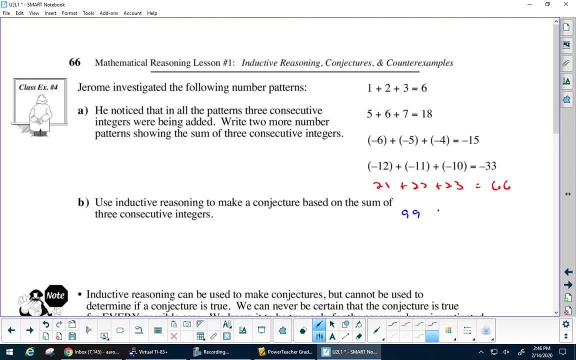 watch quick: if I gave you 99, 100, 101, what would be the sum 300? what's a fast way to do it? now, the middle number times 3, look: 2 times 3, 6 times 3 negative, 5 times 3, negative, 11 times 3, 22 times 300 times 3. right, because that one's always. 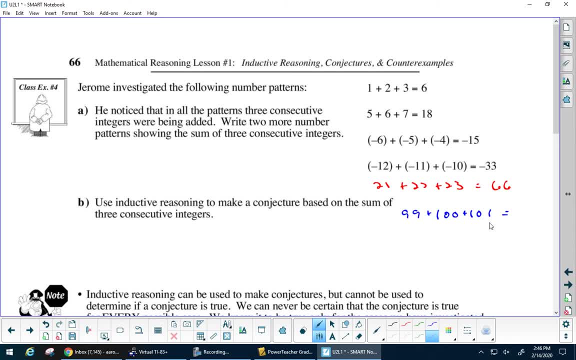 going to come here and that would be 100 plus 100 plus 100, right, so use inductive reason to make conjecture. the sum of three consecutive- now consecutive means one after the other- January, February, March consecutive integers- is equal to three times the middle integer. 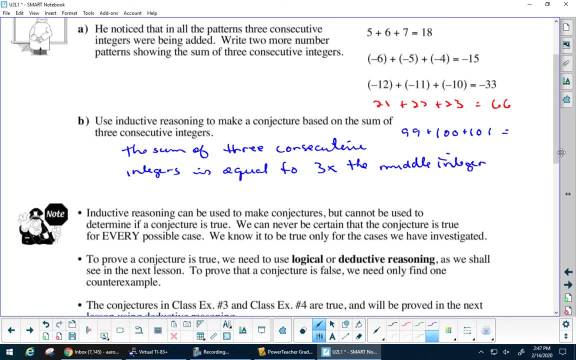 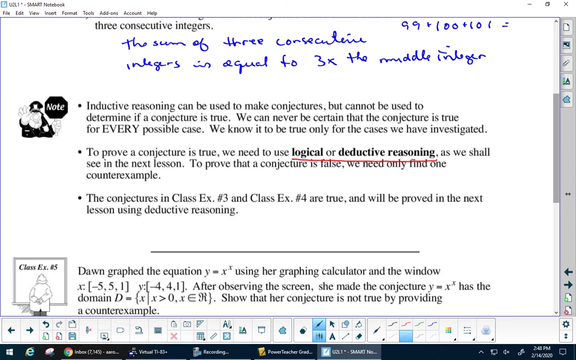 sorry, fractions, ooh. and what is the duck? oh, you now. can you give me an example where this would not be true? be true. Now we're going to learn how to prove it using logical or deductive reasoning next. Okay, so now what we want to do is: let's get out our blank piece of paper. 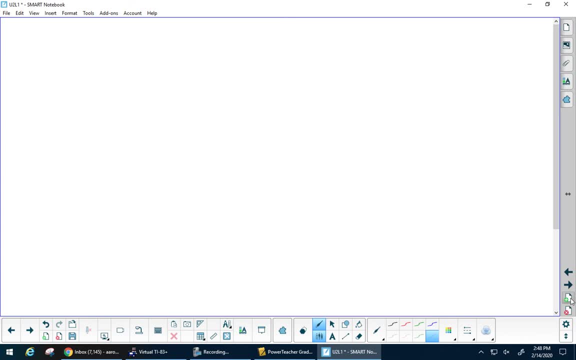 and we're going to write down what we learned today. So, because your quiz is going to be far away, So then you could just pull that out and get it all back. Okay, and I want us to be updating our study sheet every day, So at the end we've got our study sheet done. Okay, so this one. 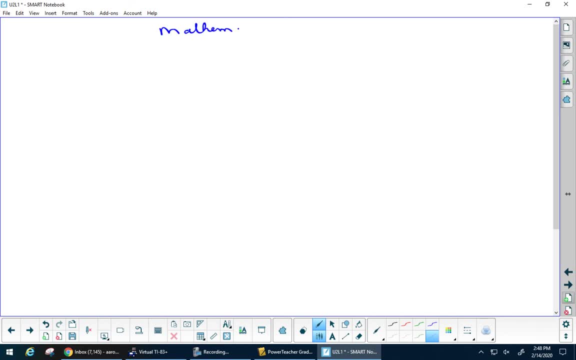 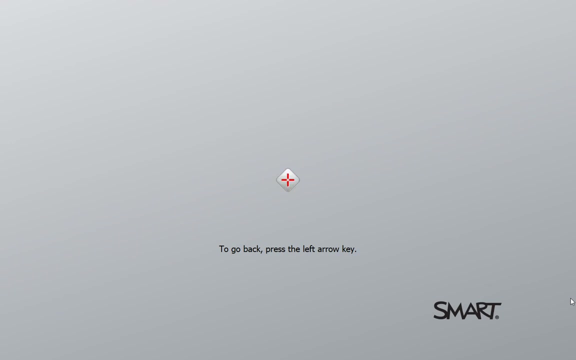 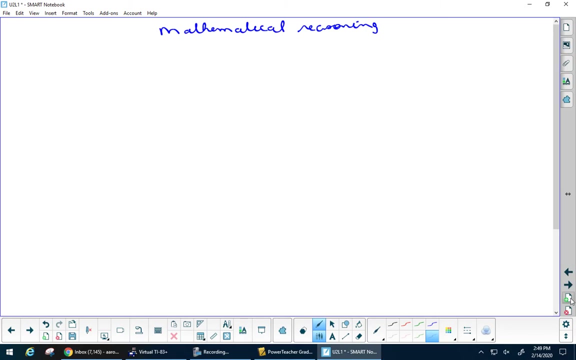 we are going to title it mathematical reasoning. No, we're going to keep that. We want to keep our sheets separate, Okay so no, we're going to keep that. We want to keep our sheets separate. Lesson one: And then we don't have to do this at the end, We're going to know it. Okay. Now, if we go back, 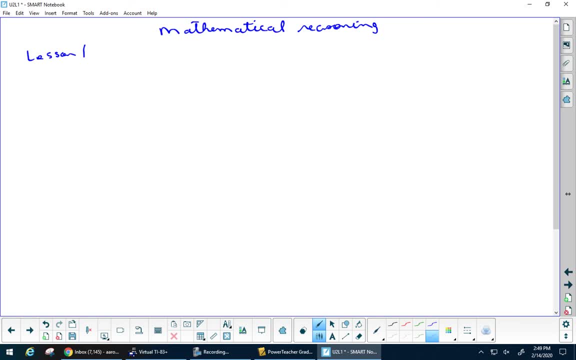 to the first page. what did we really learn there? We just did a bunch of stuff right that we just got going. So let's get our definition for inductive reasoning Right, because if we have this, then the next time we do deductive reasoning we can look at them at the same time. 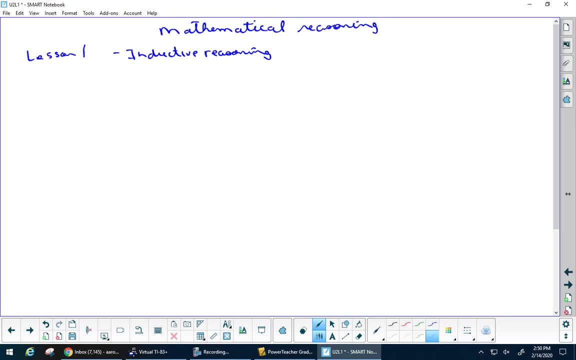 So it is a conclusion, generalization or educated guess based on experience, observations or patterns. Okay. so then let's get a conjecture. Okay, that is a conclusion from inductive reasoning. Okay, and then the last thing: a counterexample is an example which shows a conjecture is false. 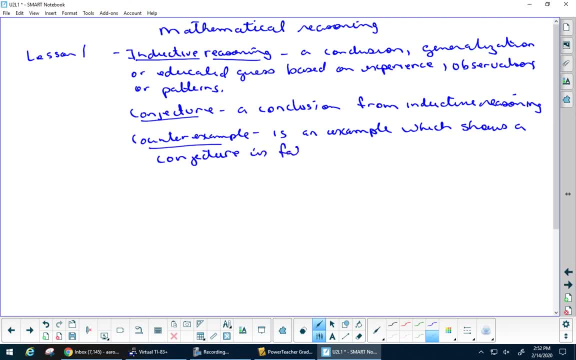 Okay, and remember, it takes just one. You don't have to provide 20.. Sometimes we want to provide 20 because it makes us sound better and we want to keep yelling, and we want to, and I did it on Wednesday and then I did this and I did this right.